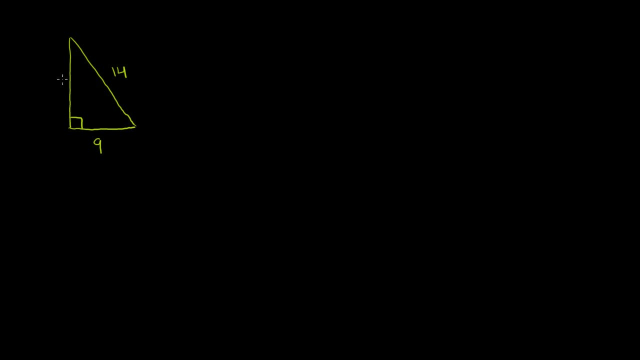 This side's length, right over here, is 9.. And we're told that this side is a And we need to find the length of a. So, as I mentioned already, this is a right triangle And we know that if we have a right triangle, 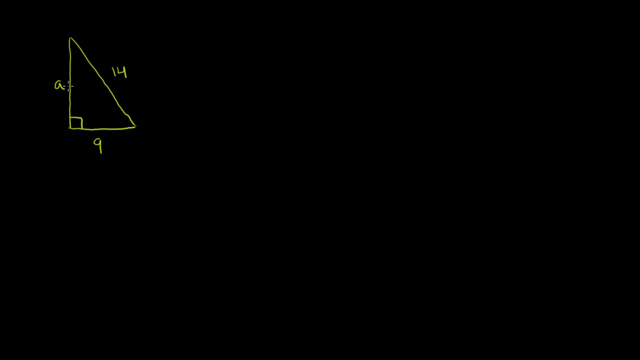 we can always figure out. if we know two of the sides, we can always figure out a third side using the Pythagorean theorem. And what the Pythagorean theorem tells us is that the sum of the squares of the shorter sides is going to be equal to the square of the longer side. 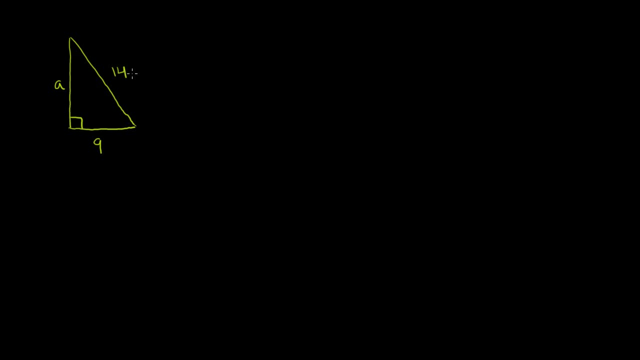 or the square of the hypotenuse. And if you're not sure about that, you're probably thinking: hey, Sal, how do I know that a is shorter than this side over here? How do I know it's not 15 or 16?? 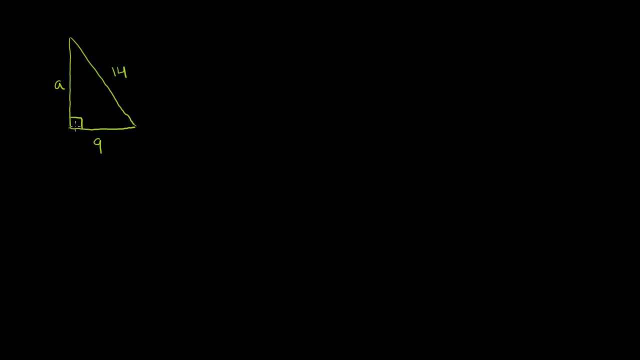 And the way to tell is that the longest side in a right triangle- this only applies to a right triangle- is the side opposite the 90-degree angle, And in this case 14 is opposite the 90 degrees. This 90-degree angle kind of opens into this longest side. 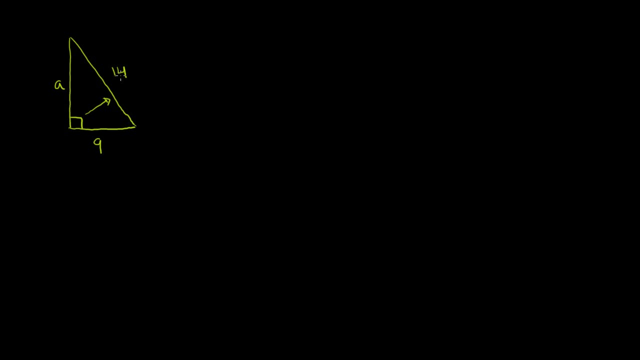 the side that we call the hypotenuse. So now that we know that that's the longest side, let me color code it. So this is the longest side, this is one of the shorter sides and this is the other of the shorter sides. 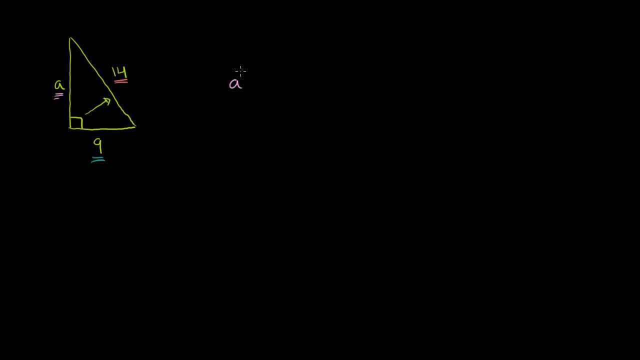 The Pythagorean theorem tells us that the sum of the squares of the shorter sides, so a squared plus 9 squared, is going to be equal to 14 squared. And it's really important that you realize that it's not 9 squared plus 14 squared is going to be equal to a squared. 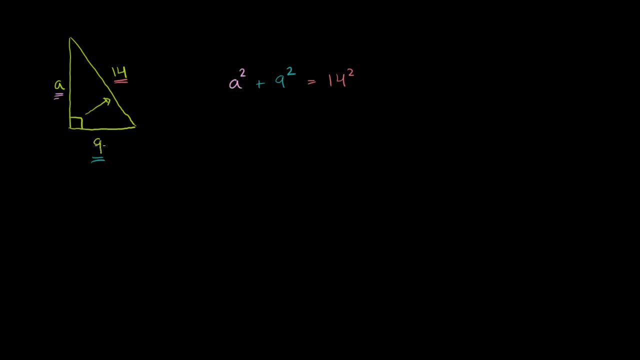 a squared is one of the shorter sides. The sum of the squares of these two sides are going to be equal to 14, squared the hypotenuse squared, And from here we just have to solve for a, So we get a squared. 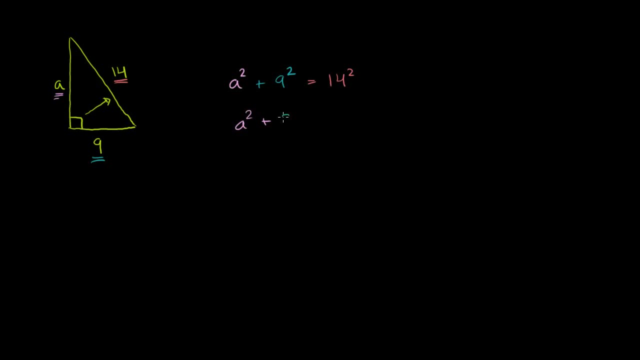 A squared plus 81 is equal to 14 squared, And in case we don't know what that is, let's just multiply it out 14 times 14.. 4 times 4 is 16.. 4 times 1 is 4, plus 1 is 5.. 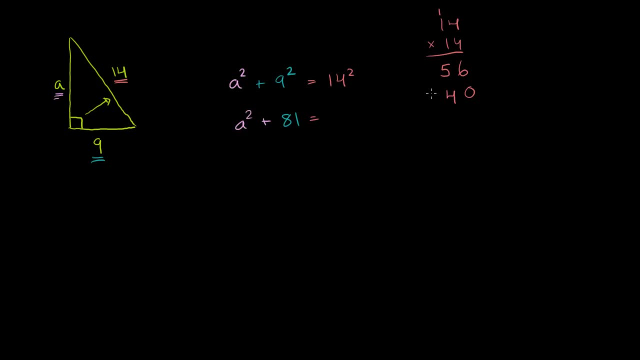 Stick a 0 there. 1 times 4 is 4.. 1 times 1 is 1.. 6 plus 0 is 6.. 5 plus 4 is 9.. Bring down the 1.. It's 196..